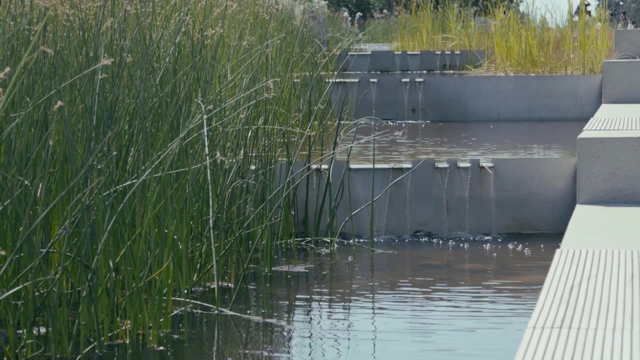 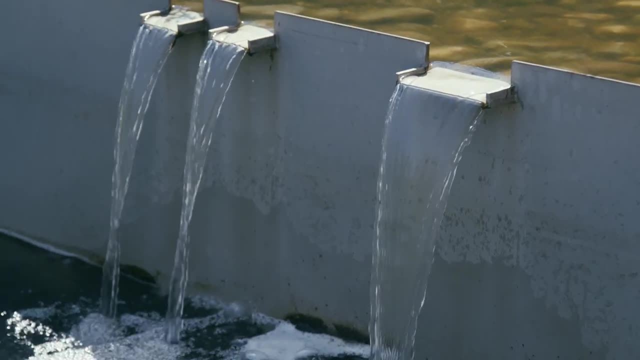 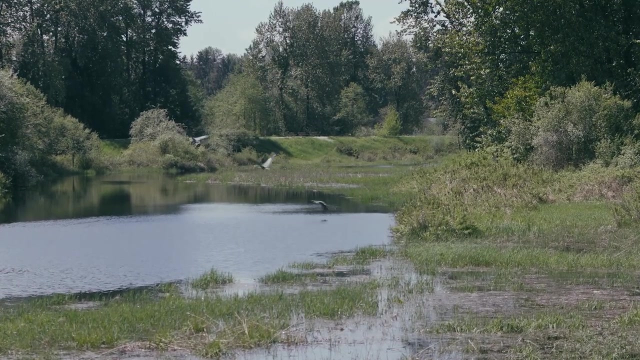 it's really looking at the environment values of green space in a more holistic manner. rather than putting it on the ground, Maybe it's putting a large or more costly pipe in the ground, Maybe it's money better spent to retain a park or a wetland that can provide that function of storing and infiltrating. 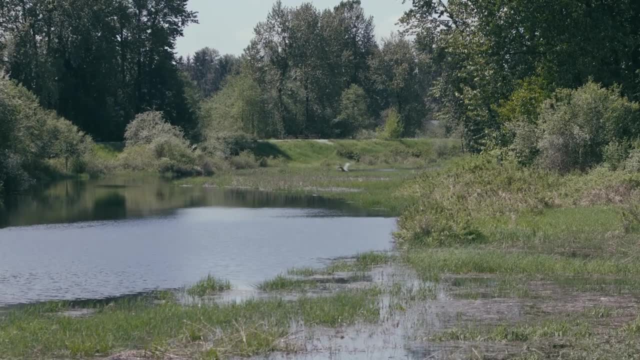 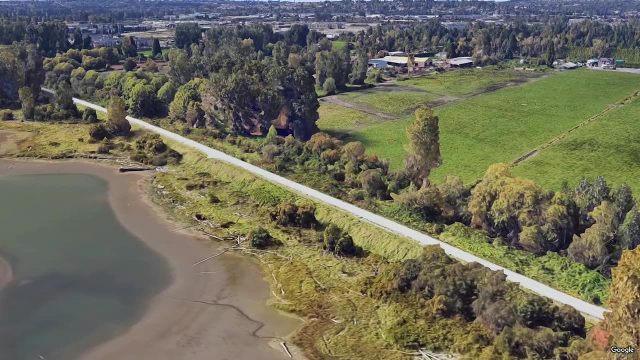 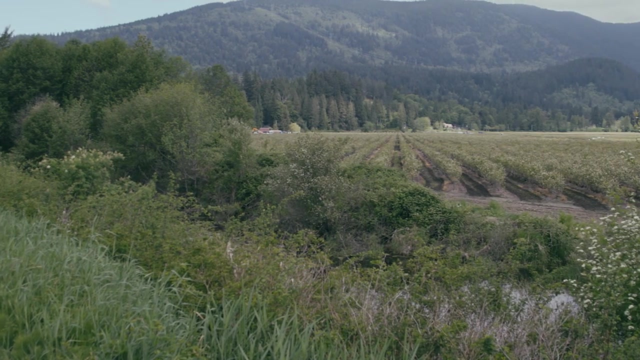 water. Much of the lower mainland is protected by a dike system. Many of the dike alignments that were constructed throughout the 60s, 70s and 80s were constructed to sort of maximize the land available behind the dikes without as much consideration to, you know, the water. 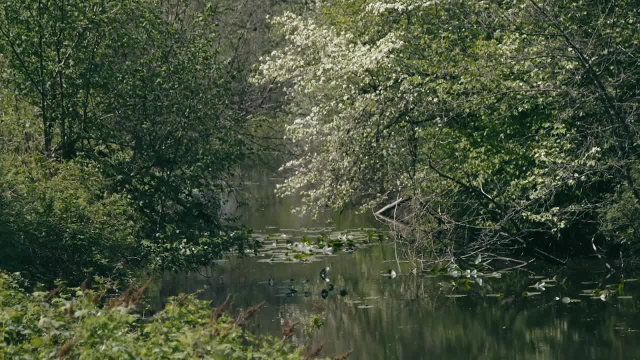 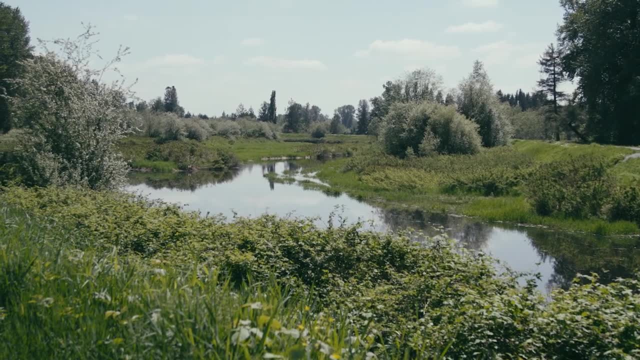 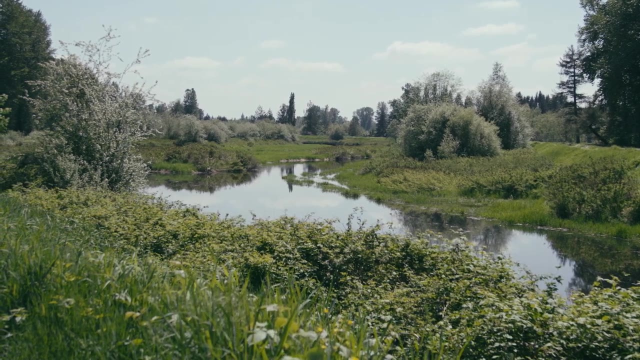 system And the reason for this is that sort of infrastructure of these dikes. the dike systems were built to provide the river room and to provide the riparian habitat, And what that did is prevented the periodic inundation and flooding of those near river areas. So there's real significant. 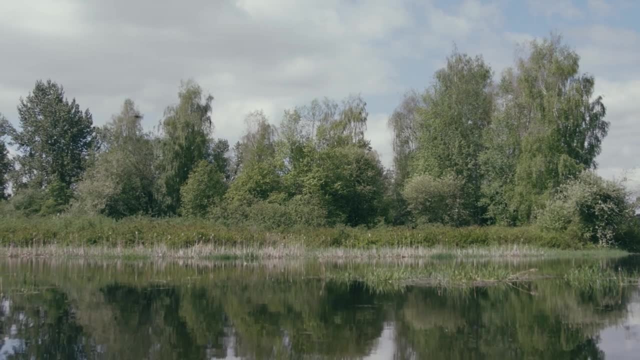 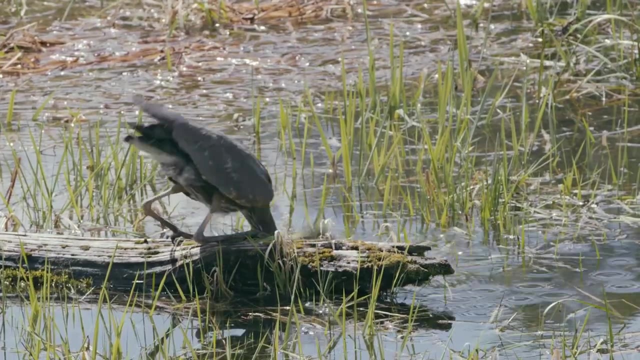 environmental benefits to that sort of flushing that used to occur. It filters out sediments, it provides potential increase in aeration, it provides habitat for fish and amphibians. So it's a lot of different things And you can see that if you're looking at the river. 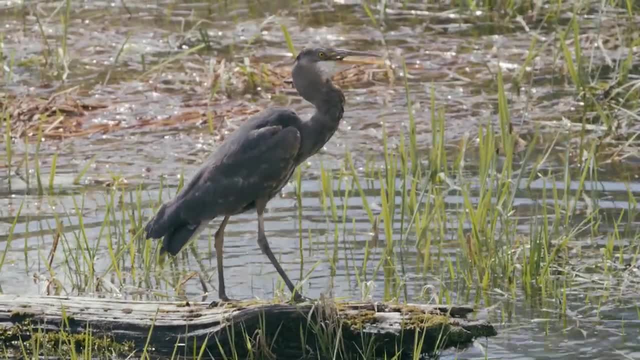 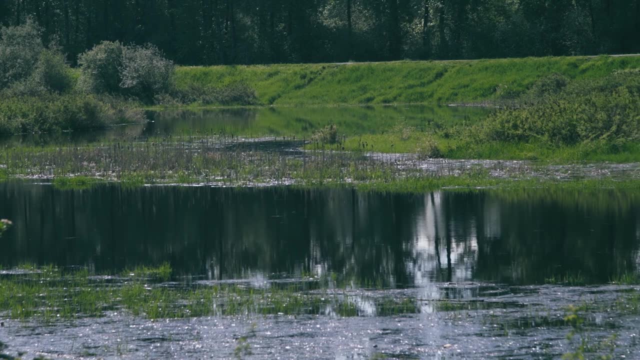 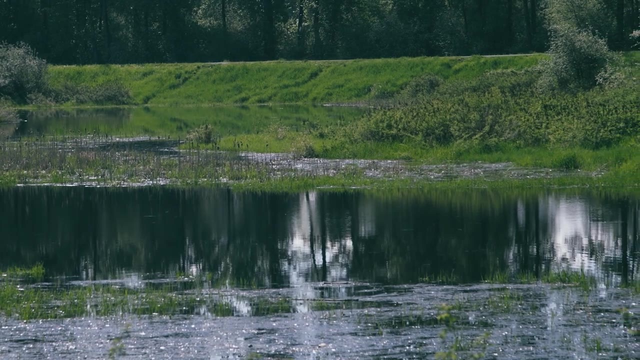 ability of the river to convey high flows and flood. So there is a bit of a trend that there's certainly a desire to set back some dikes to make more room for the river, to provide higher and improved ecological values, and there's some areas where that's been quite successful, For example in Port Coquitlam. 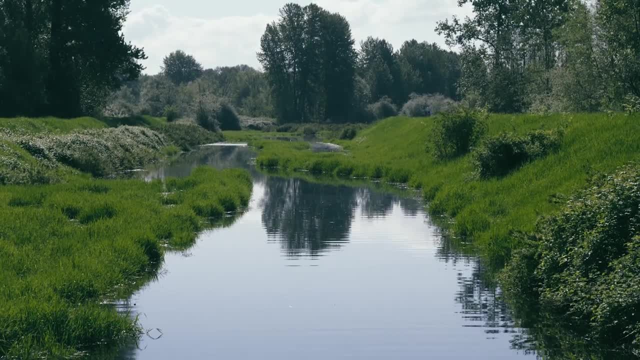 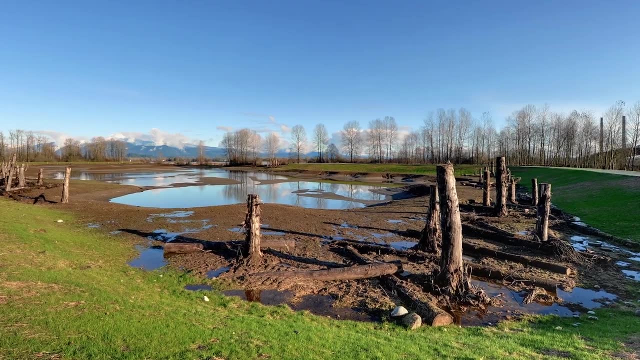 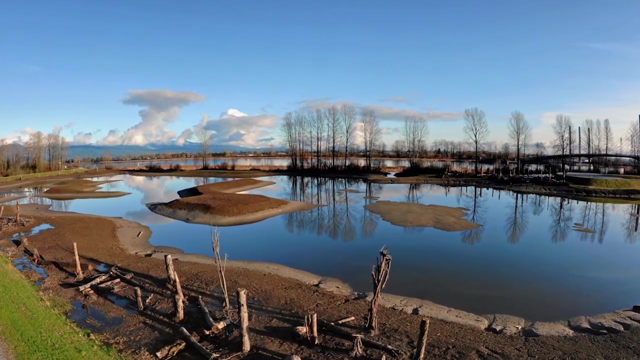 and we were able to take an existing dike that was along the riverbank and set it back approximately 150 meters, I believe, from the riverbank to allow that intertidal flushing to occur once again in those in those tidal areas. One of the 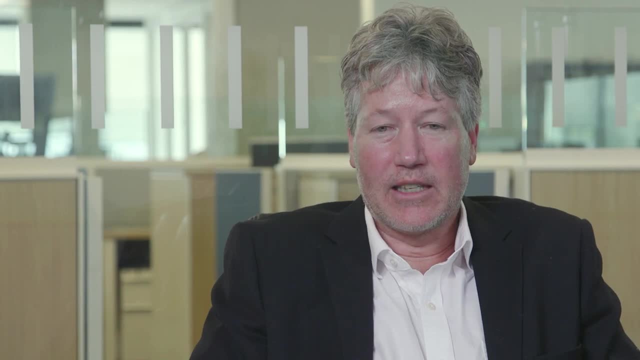 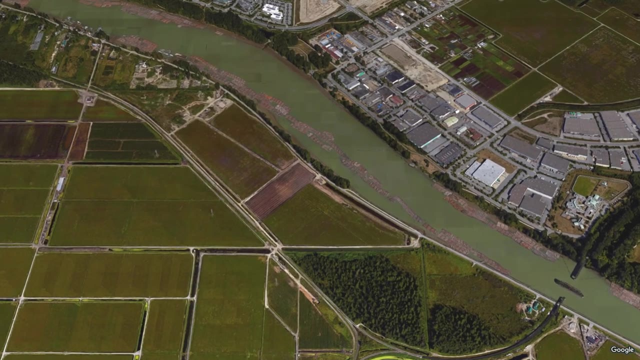 things that I think would be of real value to society is looking at more of risk-based design in terms of flood protection. Rather than setting a standard that means all areas are protected equally, it would make more sense to have the level of risk-based design in terms of flood protection. 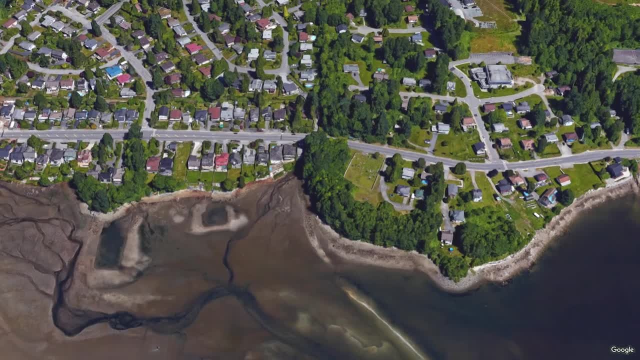 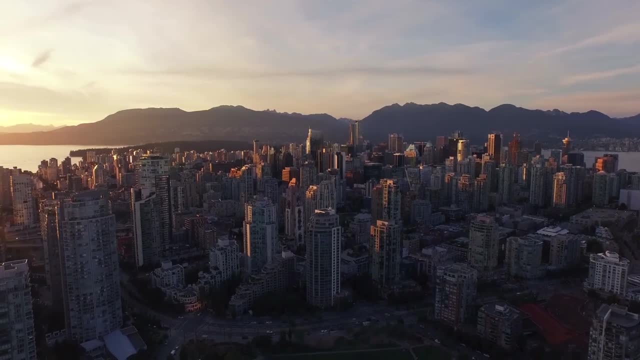 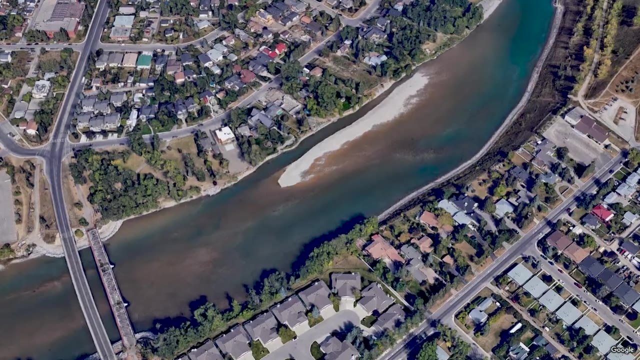 The answer is really not the level of protection related to the consequences of failure. For example, should a golf course be protected to the same level of protection, say, as a downtown core? So one particular project, we didn't just look at the financial loss, we looked at the triple bottom line. So we looked at environmental, social and